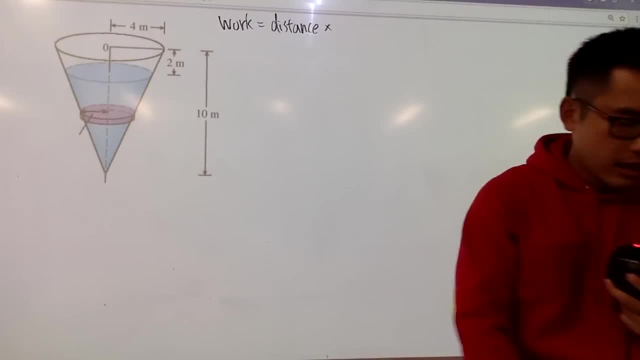 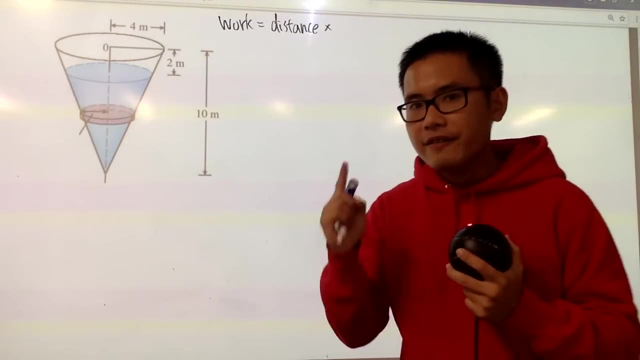 Okay, so it's distance times, force. and what is force? Force is just pretty much like the weight, right, And now how do we calculate weight? We have to care about two main things. The first thing is the density and the second thing is the volume, right? 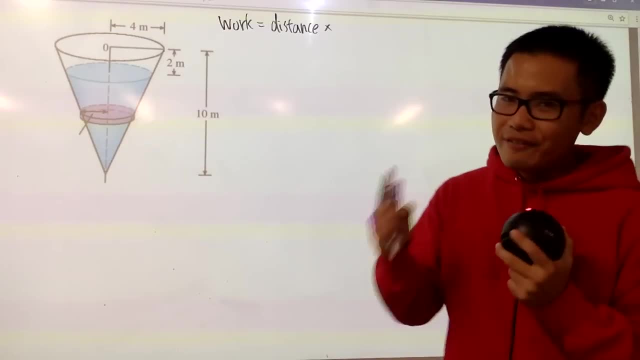 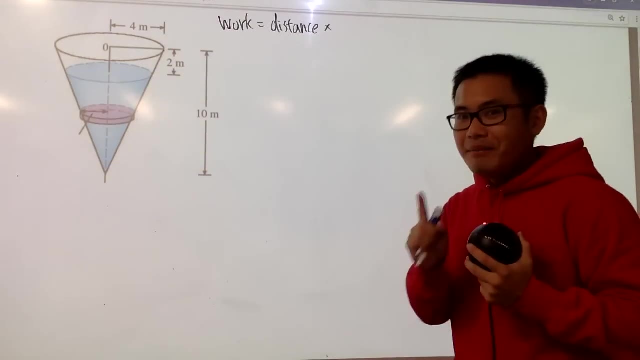 But for the density it's kind of tricky because we have two kinds of density. The first one is what we call the weight density and the other one is called the mass density. But it's kind of slightly, you know, bizarre. Let me just write down density, okay. 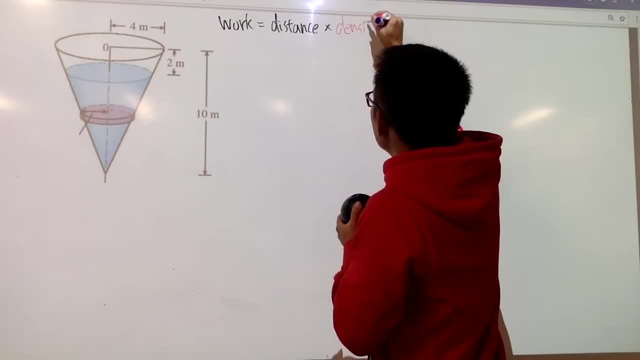 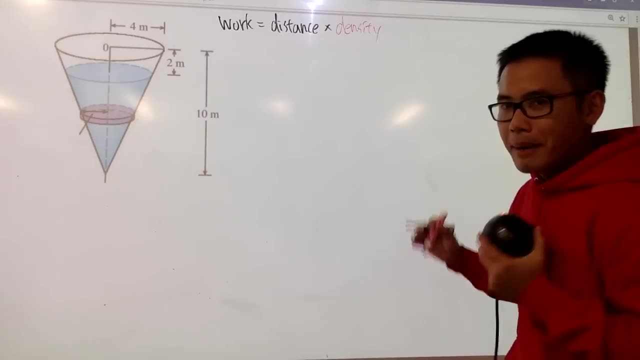 So distance times, density And I know, if I just Let me just put this down, If you guys don't watch my whole video, if you guys don't listen to what I said, you will argue in the comment section that this is not correct. but you know what It's okay. 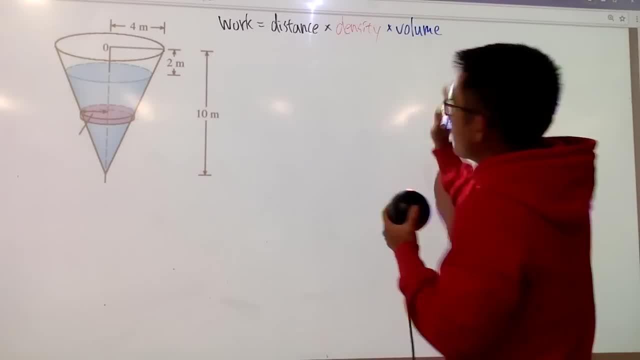 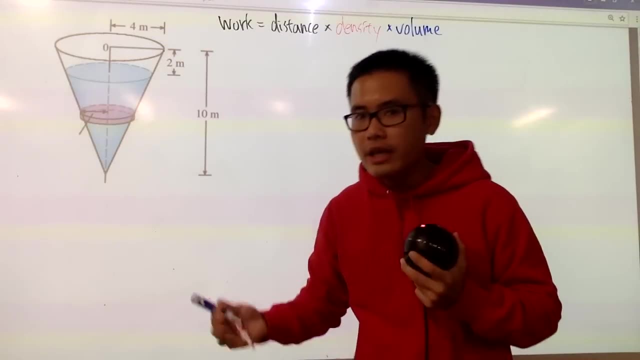 Density times volume. This right here will calculate the weight. but we have to be careful with the density part Especially. you have to pay attention to what kind of units are we in Right here. let me just indicate this for you guys. 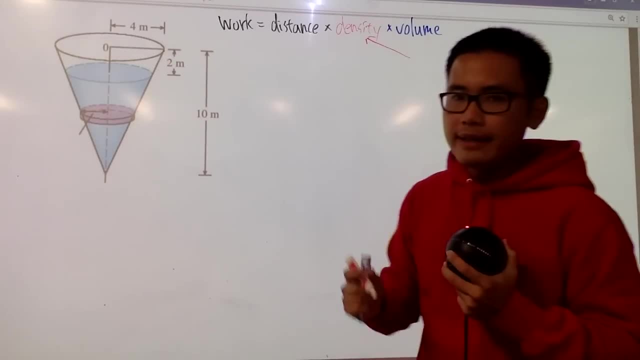 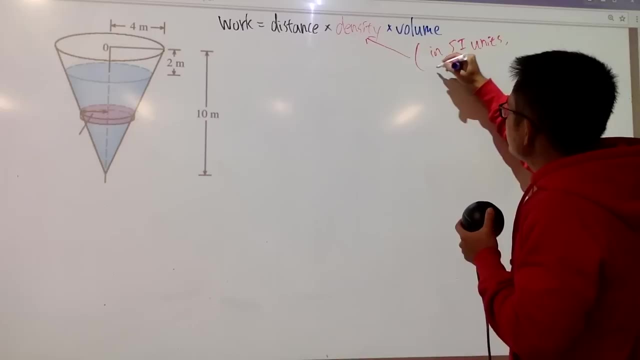 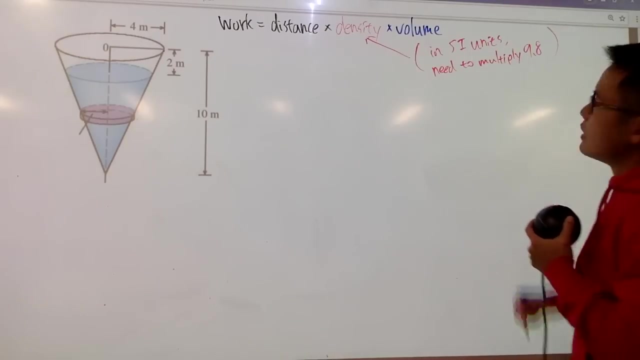 In this case, we are using meters. That means we are in the SI units, and whenever we are in the SI SI units, be sure that we need to multiply the 9.8,. okay, Well, of course that's for the gravity, but in this case that would be the mass density. 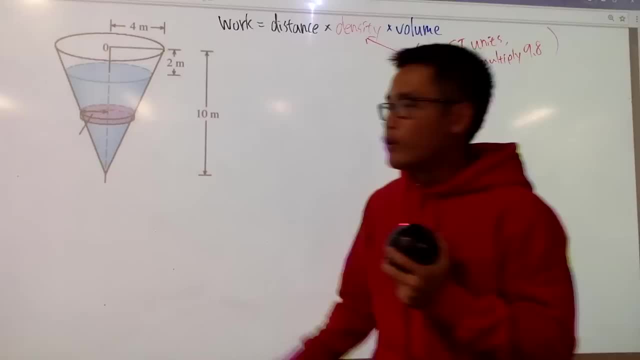 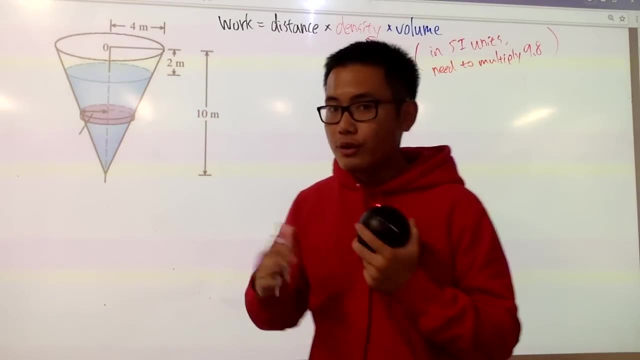 But once again let me just put down the density right here. If we're using, let's say, 2 feet, 10 feet, 4 feet, if we are in the US unit, we don't have to multiply by the 9.8,. 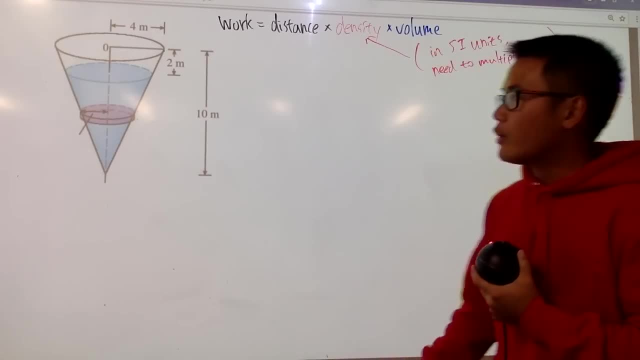 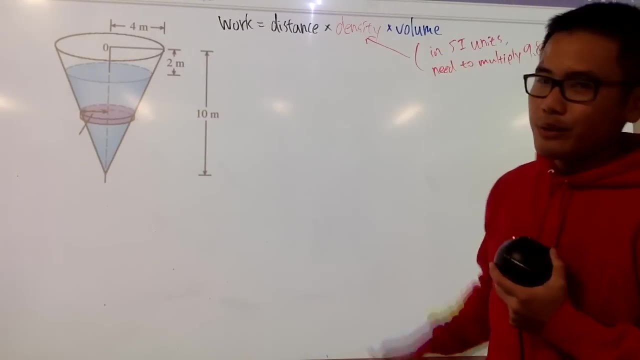 because that would be considered the weight density already. right, But remember we are pumping in water, so you also have to know the magic number, which is 1,000 in the SI unit for the mass density of the water. Anyway, here we go. 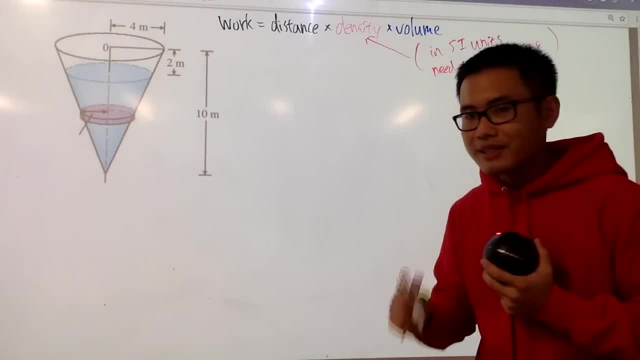 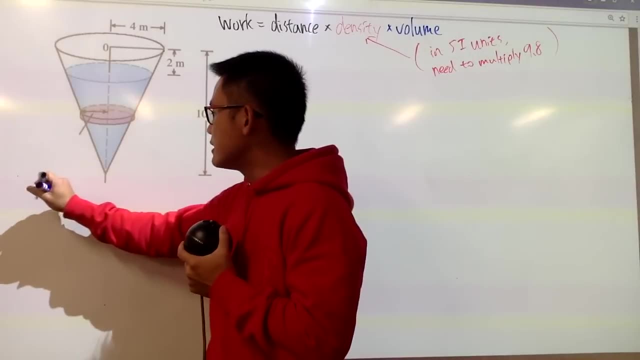 Let's figure out the volume first. okay, That's usually the hardest part, because you have to do geometry, you have to do some algebra And in order for us to do the volume, we have to come back here and I'm going to set up a reference frame. 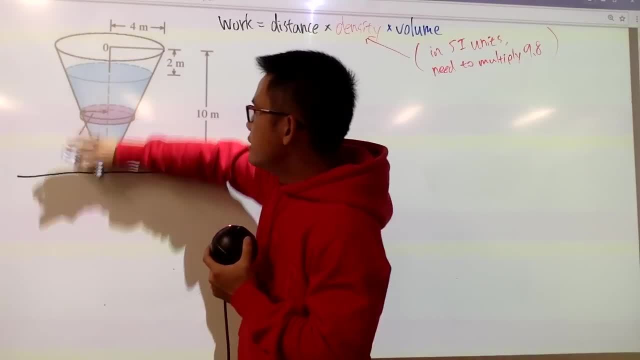 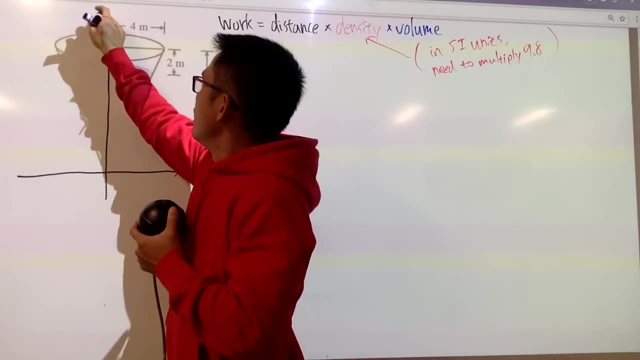 and let me just put on the x-axis down below here so that everything will be So, everything will be positive, and I will put the y-axis right in the middle like this, okay, And the style is: we'll make a horizontal cut. 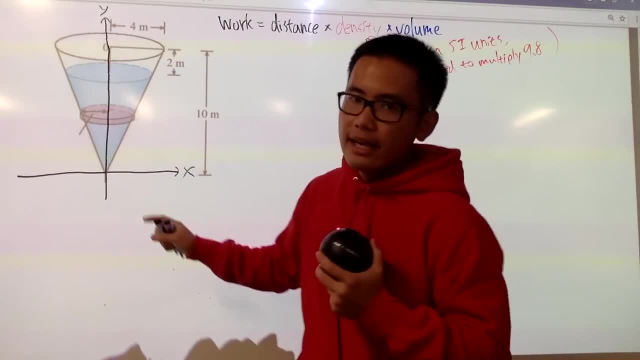 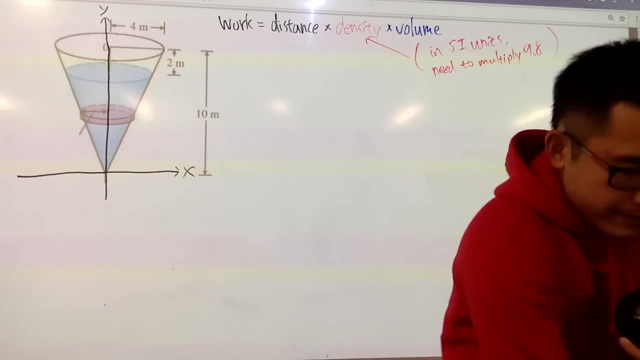 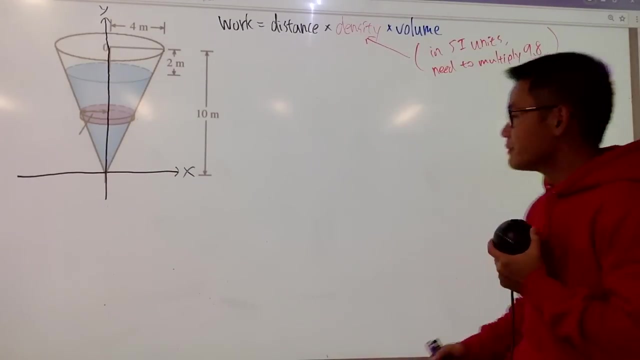 And because this was a cone, once we make a horizontal cut, as you can see, we will have a cylinder right. This right here is a small disc and it's arguably a cylinder, just like a CD right. It's pretty thin and we have to first recall that. how do we find out the volume of a cylinder? 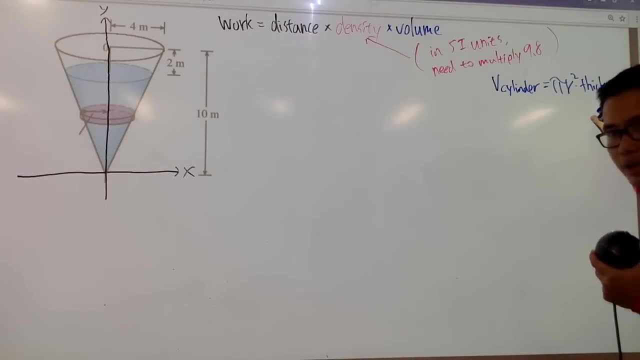 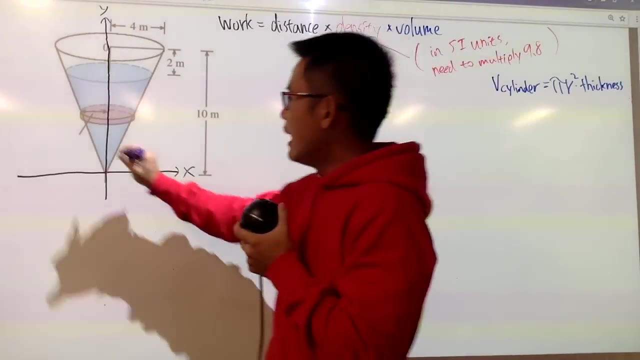 And Now we'll figure out everything. from right to left, The thickness is equal to the differential. okay, Either the dy or whatsoever. So we come back here. as you can see, here is the small cut that we made, right. 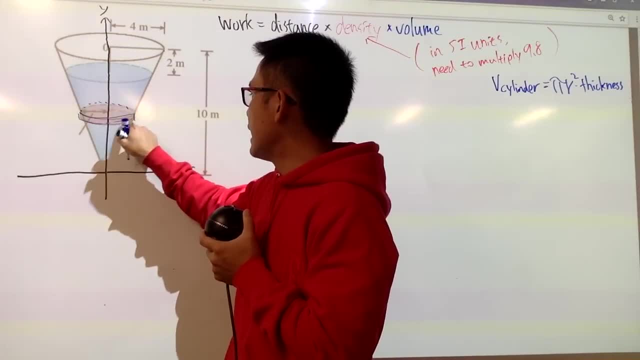 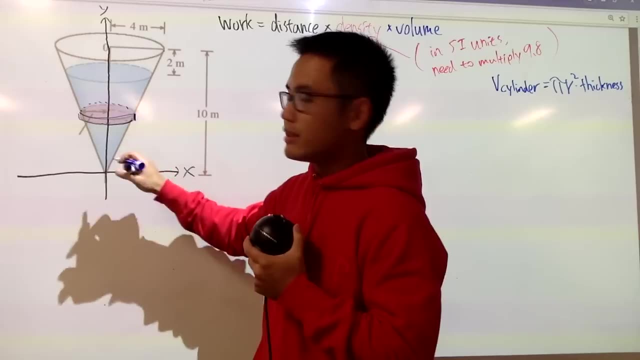 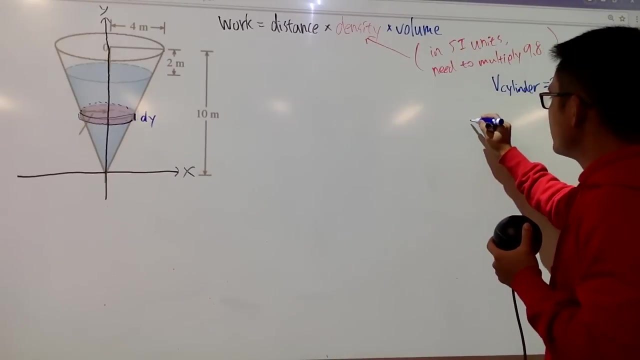 It's just a small disc and you will see that the thickness right here is just a small change in amount in the y-axis right. So this will be denoted as dy and that's the thickness. Now let's figure out the volume. so let's put down dy first. 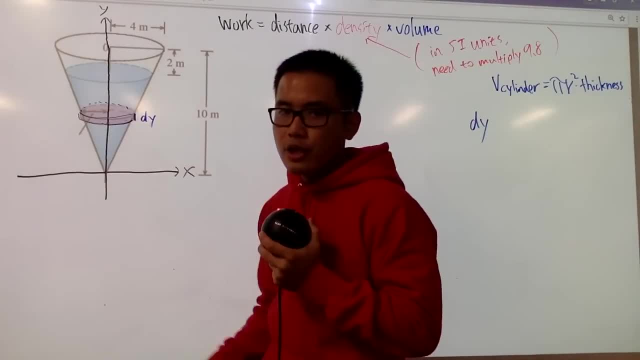 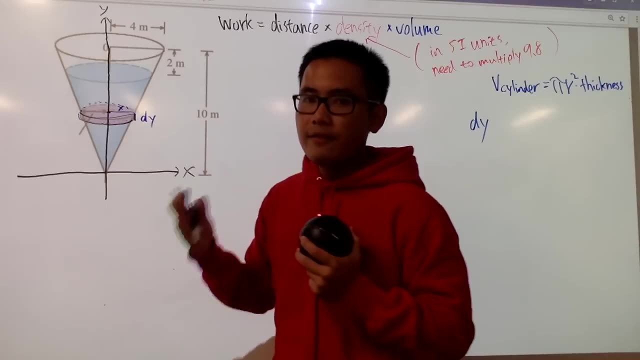 Next, I have to figure out the radius. Well, based on this picture, as we can see the radius of this disc, it will be from here to here which is going to be the x value, because that's the horizontal distance. okay. 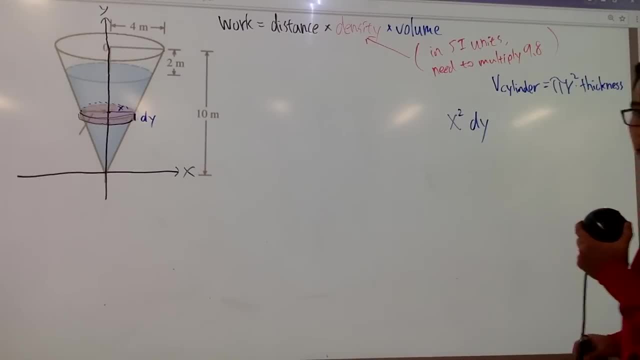 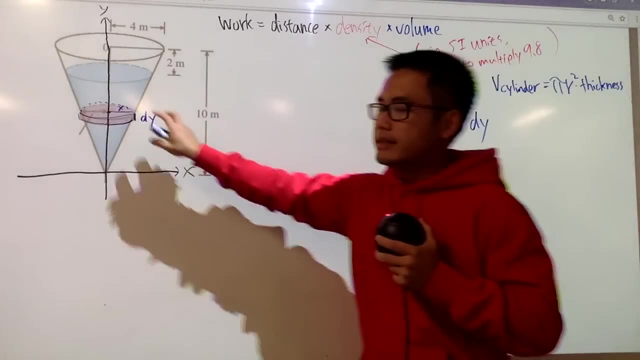 So the radius is x, so we will have x squared, and then next, of course, we will multiply it by the pi, and now this right here represents the volume of this disc. We are not done yet, but let's just continue, okay. 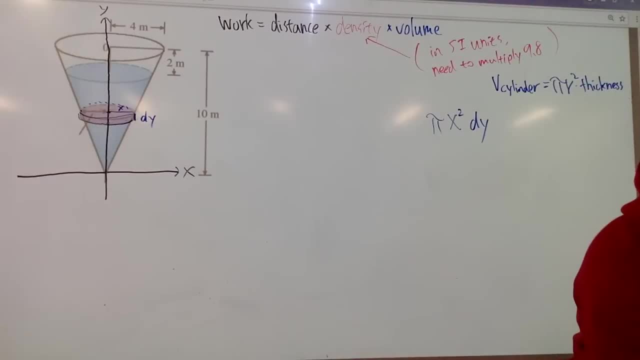 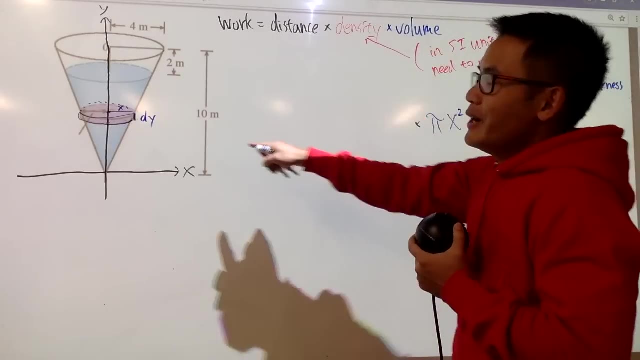 Next, we are going to figure out the density. How can we figure out the density? Well, it's just some constants that you have to look up. It depends on what kind of things that you have. okay, Right here we are talking about water. so the mass density of the water is 1,000,. 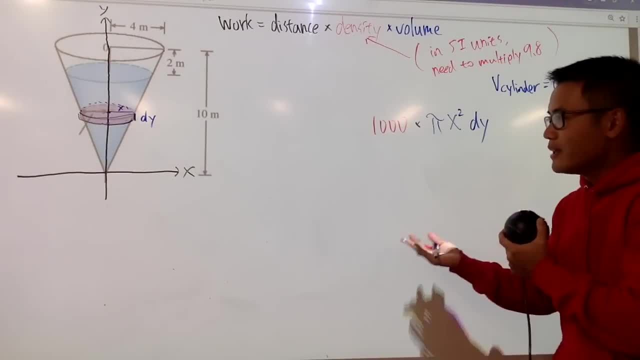 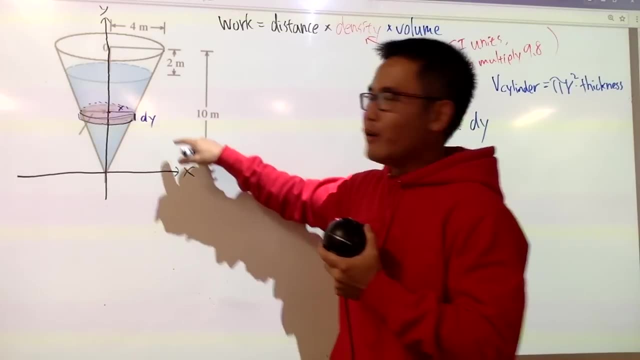 and let's not put down any units yet. as long as you are making sure that all the units are good, you'll be okay, As long as you don't have, let's say, 10 meters. and then all of a sudden you get like: 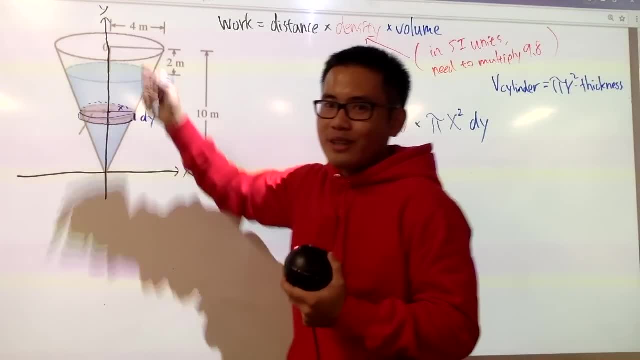 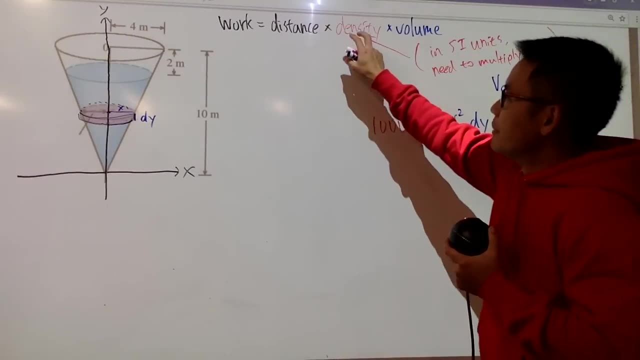 2 centimeters and all of a sudden you get like 4 yards or whatsoever. that will be a pretty messed up situation, but usually that won't happen, okay, Anyway, so the mass density of the water, that's water, not gasoline or not milk or whatsoever. 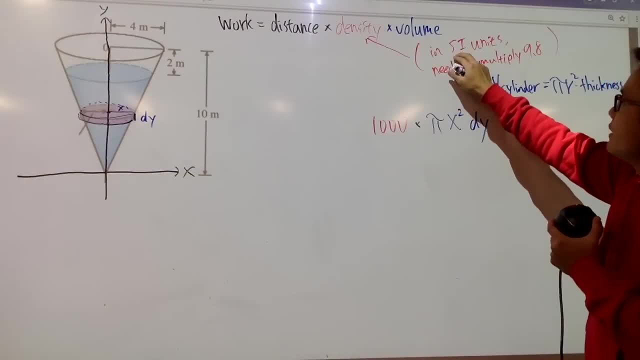 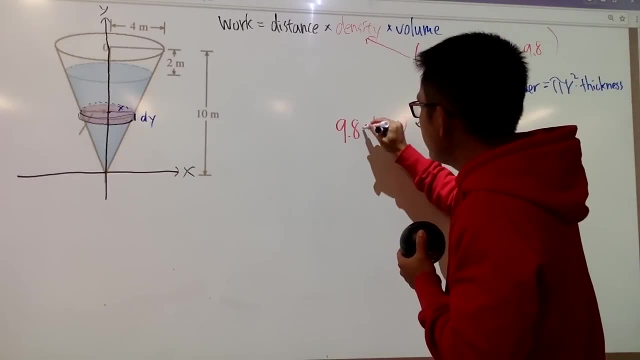 it's 1,000, right for water. and once again, whenever we are in the SI unit, we have to remember to multiply by 9.8 because of the gravity. okay, So we multiply by 9.8, so this right here will take care of the density part. 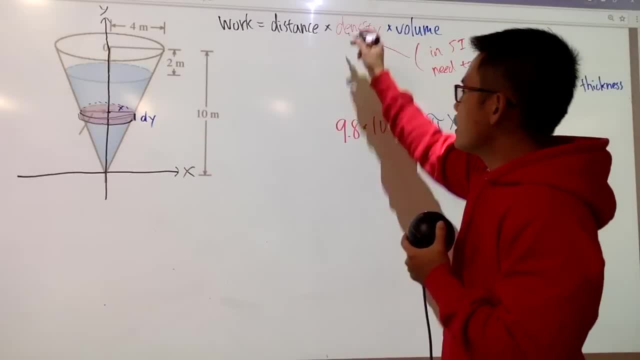 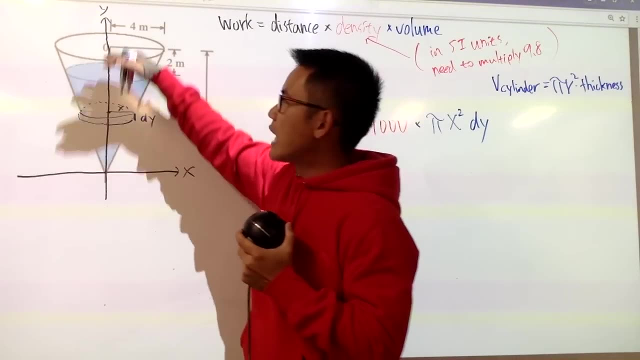 of whatever we have in the tank. Next, we are going to figure out the distance. For the distance, it's the following: We have to figure out the distance from here all the way to the top of the tank so the water can be out. 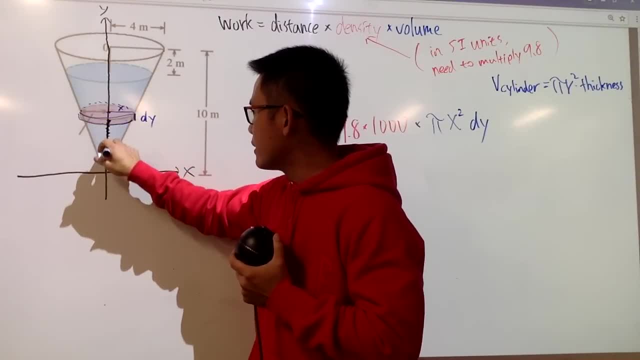 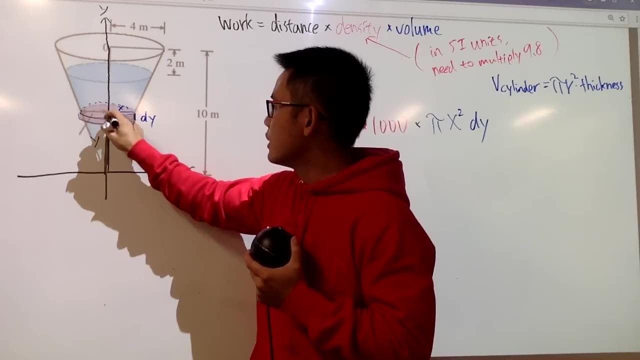 Well, based on this picture that we have, the distance right here, right from here to here, is the y-value, because that's the vertical distance. The horizontal distance was the x. okay, But I care about the distance from here to here. 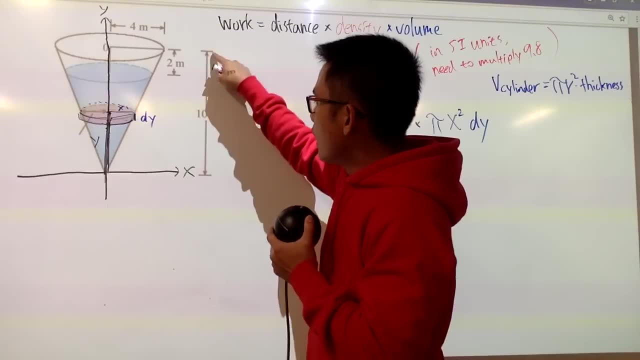 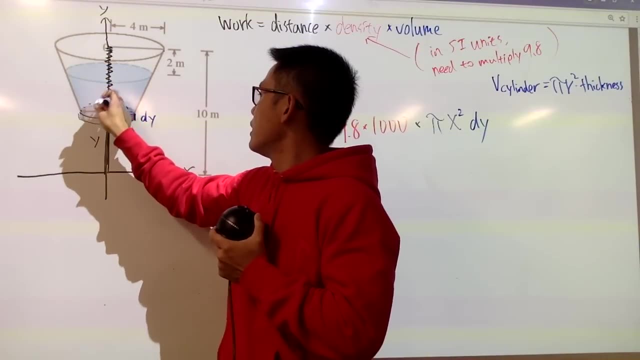 so that the water can be out. It can be out, okay. Well, the whole thing is 10.. This much is y already, which implies that from here to here, the distance is just 10 minus y, isn't it? 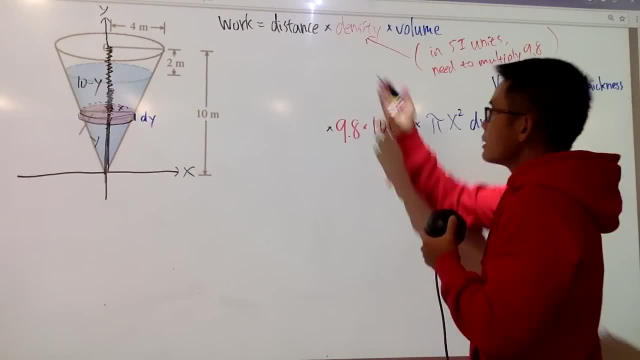 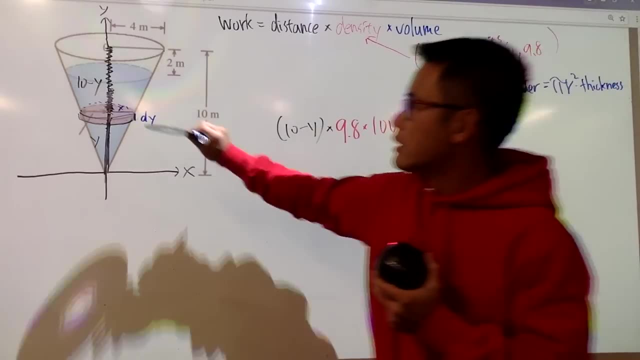 So let me write this down 10 minus y, and we multiply by 10 minus y right here. This represents the work that we need to pump out this much of the water from here to the top of the tank. okay, And how many of these kinds of things do we have? 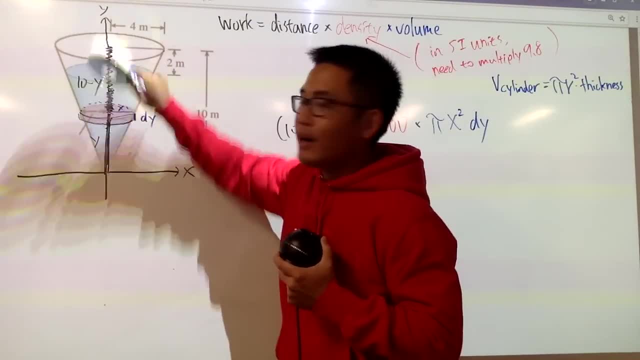 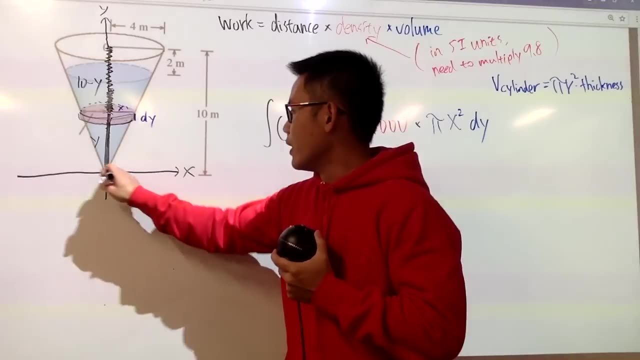 A lot. Here is the first one, All the way up to here. This is the time we have to integrate, to add them up. okay, So we integrate over. well, the y-value of here is 0.. Up here- originally it was 10 for the whole thing. 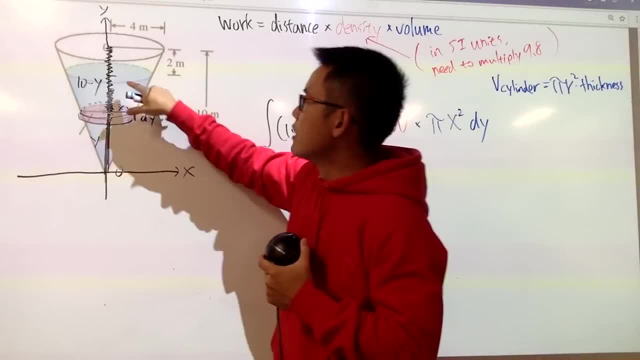 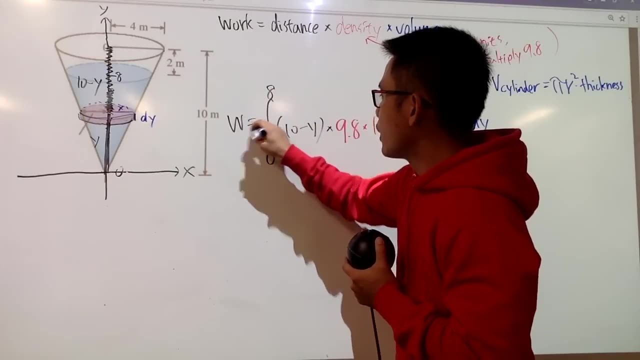 but the first 2 meters on top is empty. So from here to here is only 8.. Therefore, we have to integrate from 0 to 8. And this will pretty much become 0.. Okay, calculate the work for you. Unfortunately, notice that X is not invited in the Y. 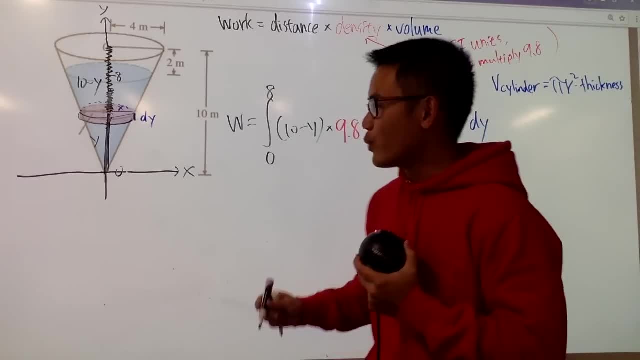 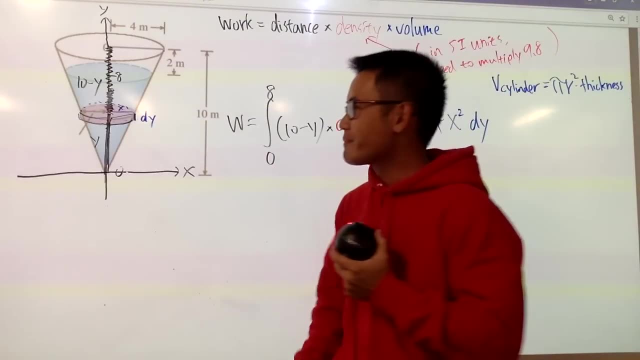 world. so we have to do more math, okay, And here is where the X and Y axis comes in, because we can do some- you know geometry by using algebra. okay, If you look at this picture on the side here, this is just a straight line and of 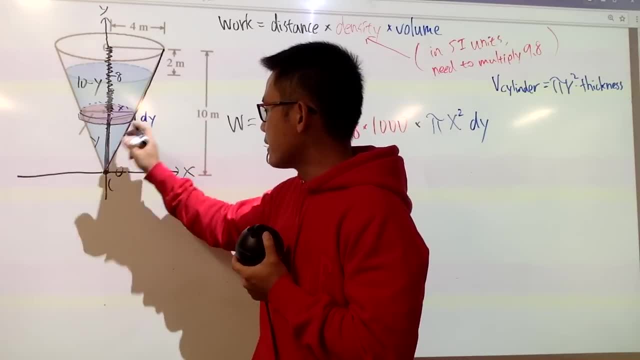 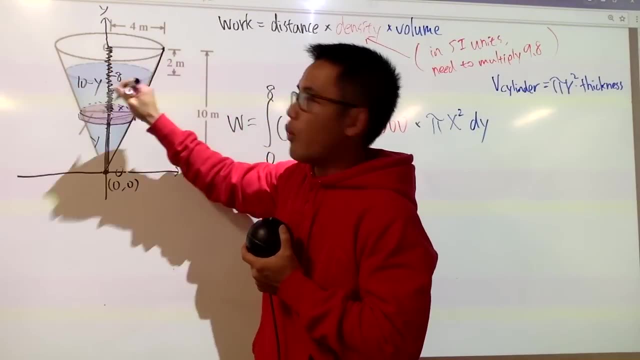 course, we know how to find an equation of a line. This point here, based on the choice of our reference frame, is 0, 0, and then this point: as we know, from here to here, the X value would be 4, and then the Y value is, from here to here, which? 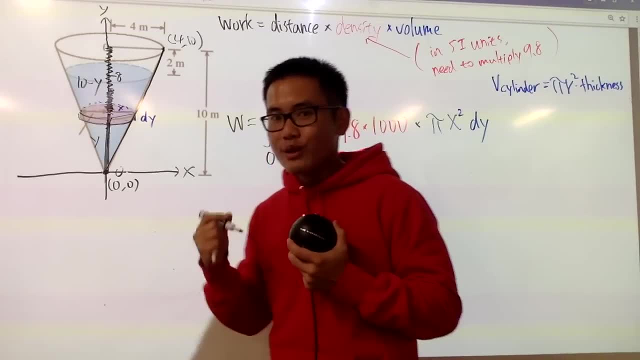 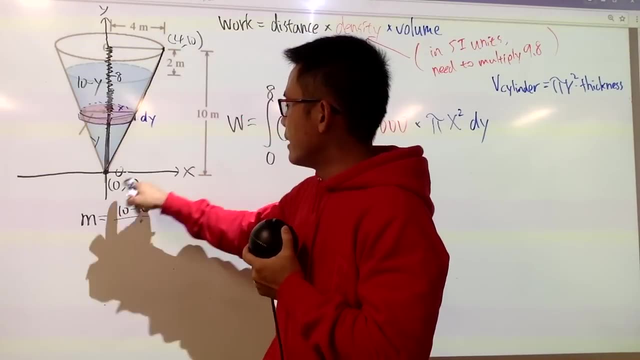 is 10, so that's 4 comma 10.. Of course we have to get a slope first, so that's M equal Y2 minus Y1, which is 10 minus 0, over X2 minus X1, which is 4 minus 0, 10. 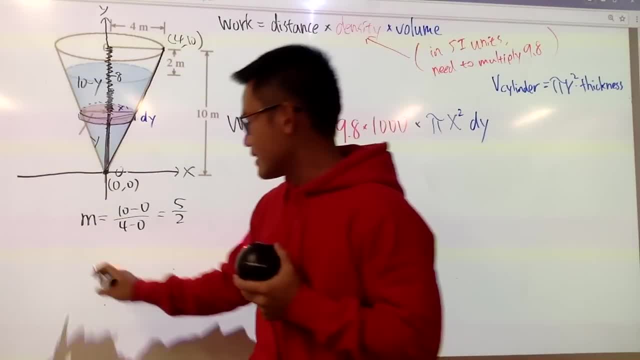 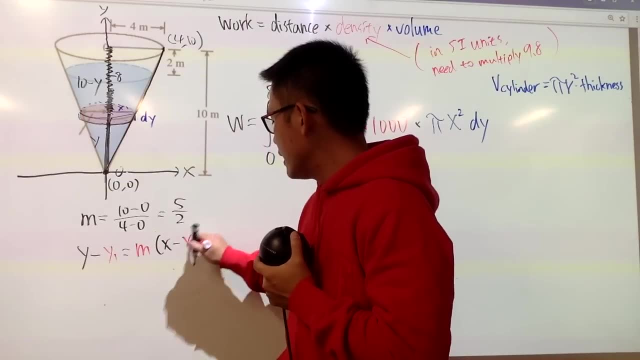 over 4, pretty much, which is 5 over 2.. And then next we can use the general equation Y minus X2 minus X1, which is 4 minus 0, and then next we can use the y1 equal to m times x minus x1. and i know i could have used: y is equal to max plus b. but let me tell. 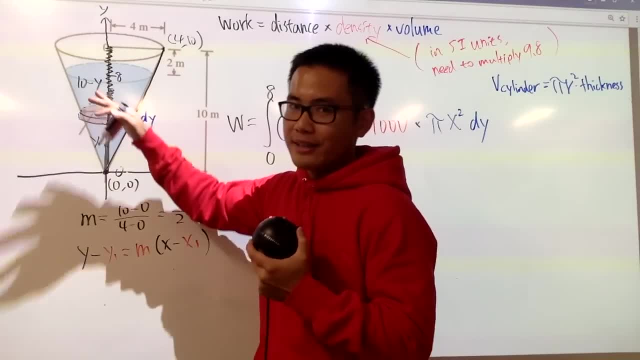 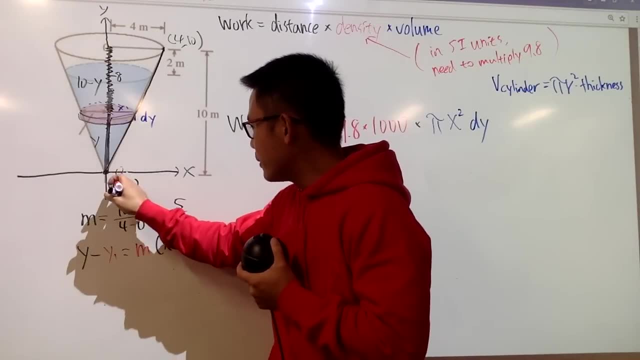 this right here will cover everything, especially if you don't get like a nice cone, maybe just a half of the cone like that, all right, so i like to just show you guys this for consistency purpose. anyway, let me label this one as x1- y1. so now you see, y is just y minus y1, which is 0. equal m is. 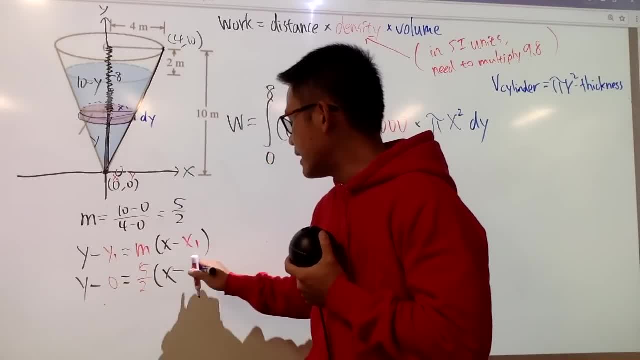 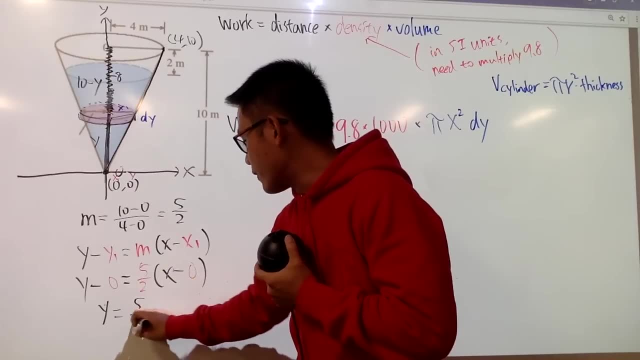 5 half times x is just x minus x1, which is 0, and now this is just y, equal this times that only, which is 5 over 2x. right, but i want to isolate the x, so in another word, x will be after we multiply. 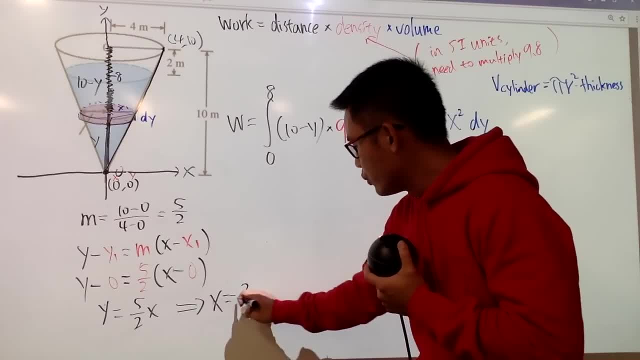 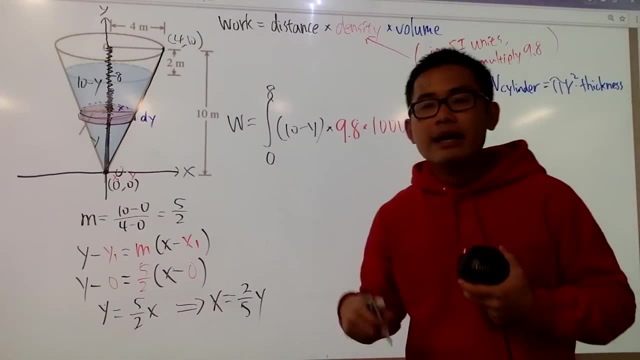 both sides by 2 over 5, we get x equal 2 over 5x. and now i will just have to plug in this into this x and i will be done for the setup and you guys will do the work of you know, maybe you. 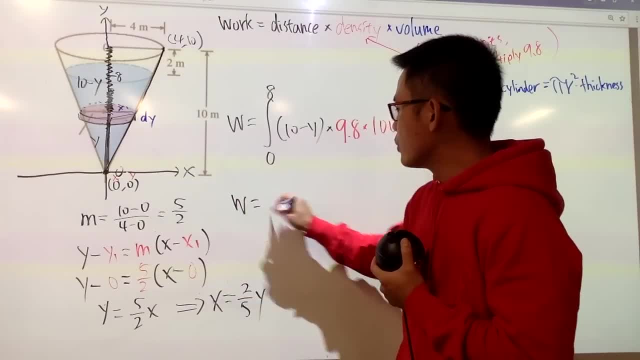 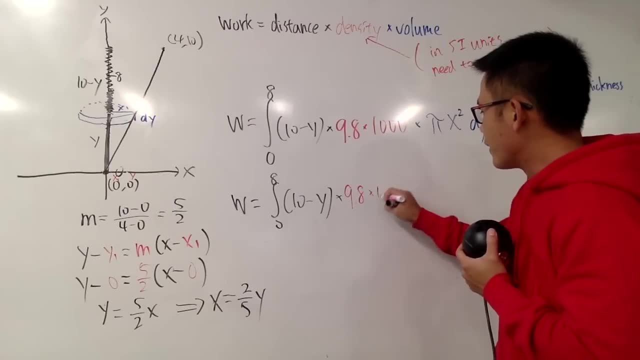 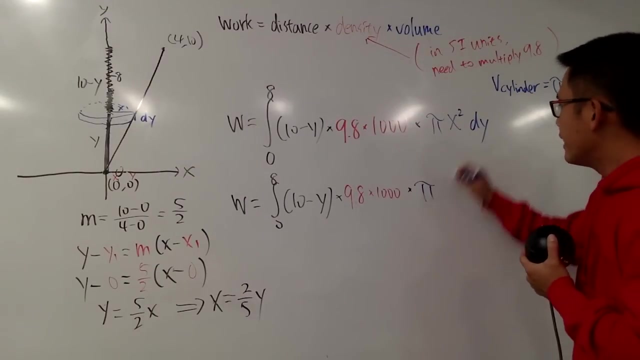 the calculator will do it by hand anyway. work is equal to from 0 to 8, 10 minus y times 9.8 times 1000, and then multiply by, we have the pi is still pi, and then for the x, we are going to open the. 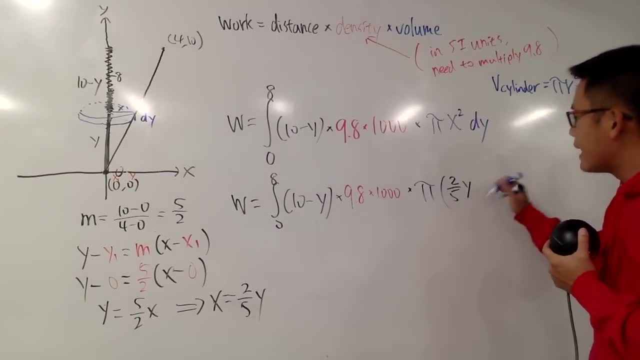 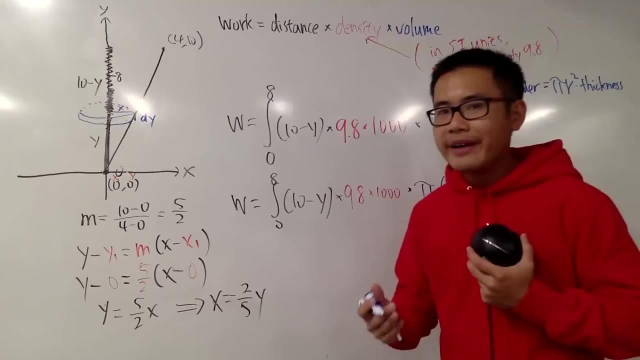 parentheses and put this in, which is 2 over 5 y, and then square that. at the end we of course have this dy. this integral will calculate the work for you, but you also have to do the work on your own to figure out the value for this leave. 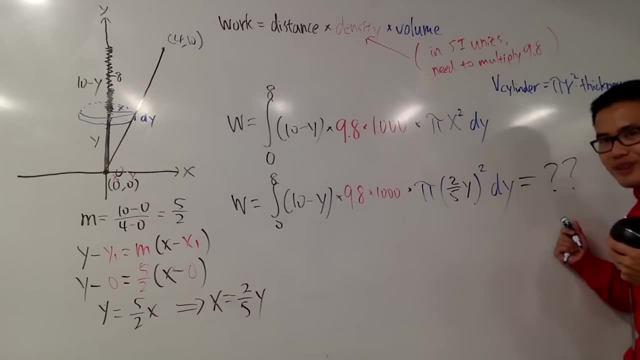 a comment down below. whoever commented correctly first, i will pinch your comment and congratulations for that. anyway, that's it.